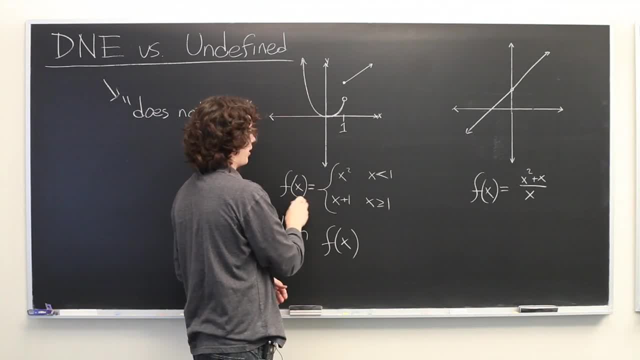 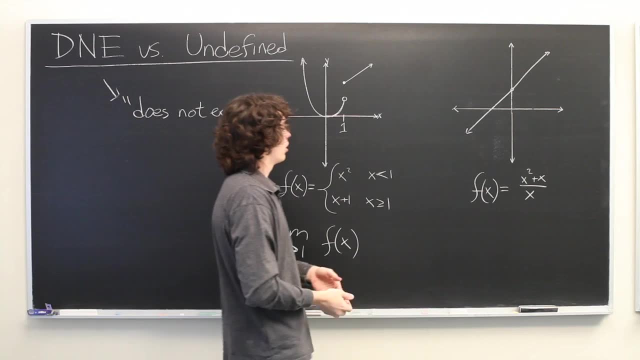 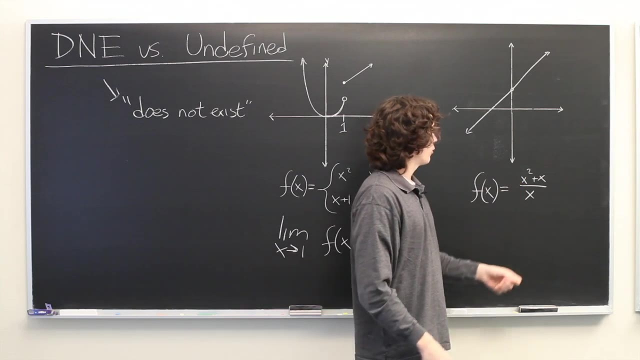 defined. at this point The function is actually defined. at this point The function is actually defined. at this point We can put in f of one and get a definite answer. So here, in this case, DNE does not imply undefined. Okay, let's look at this next example, where we have f of x equals x squared plus x over. 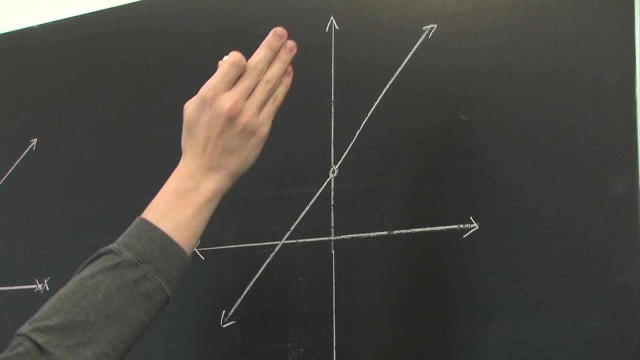 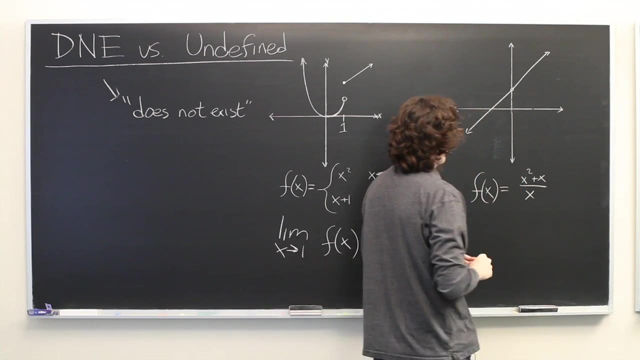 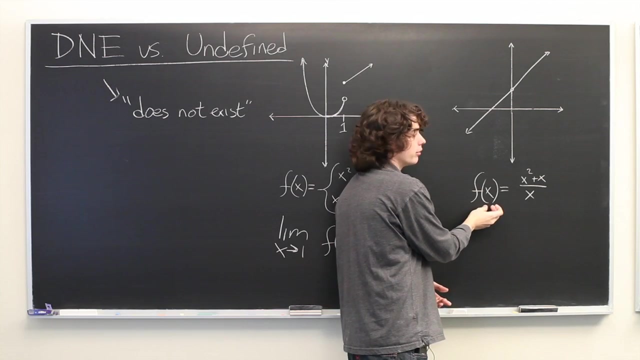 x. This essentially just gives us the line, but there is a hole or a removable discontinuity at x equals zero. At this point the function is said to be undefined. So we're going to be undefined because if we plug in f of zero, we get a zero in the denominator, And we can't. 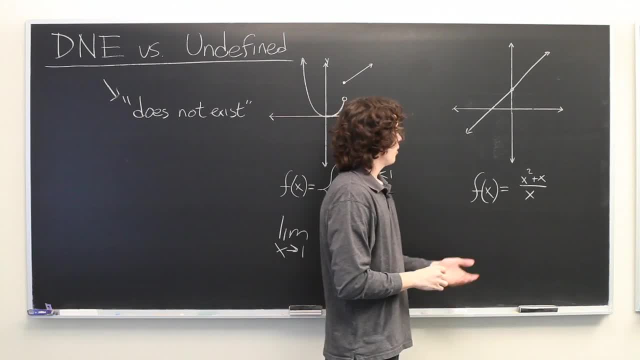 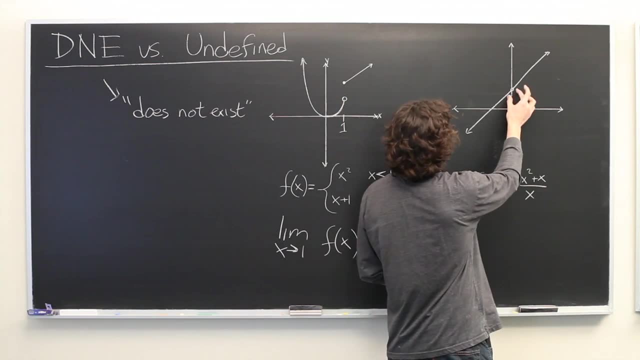 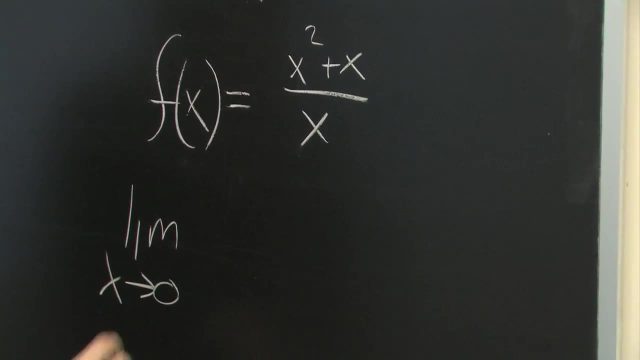 divide by zero, because that is undefined. However, in this case, undefined does not imply that the limit does not exist. It is, in fact, quite simple to compute this limit. So if we wanted to see what is the limit as x approaches zero of x squared plus x over. 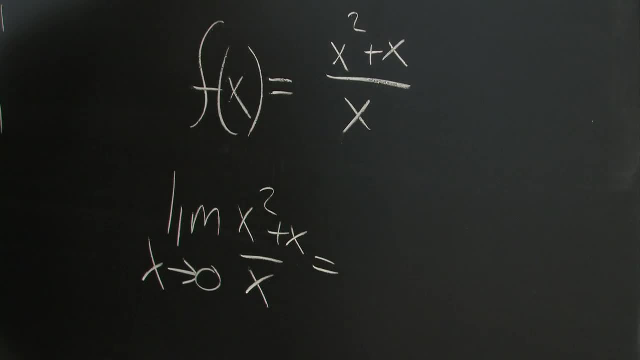 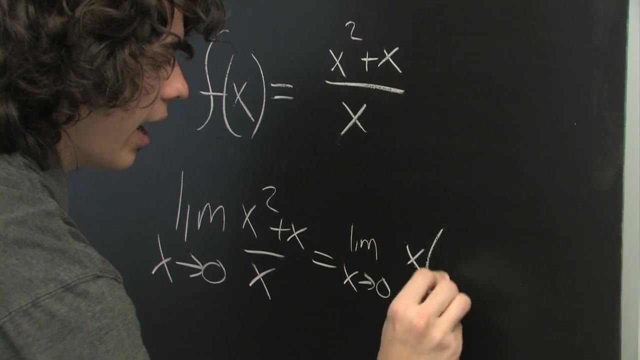 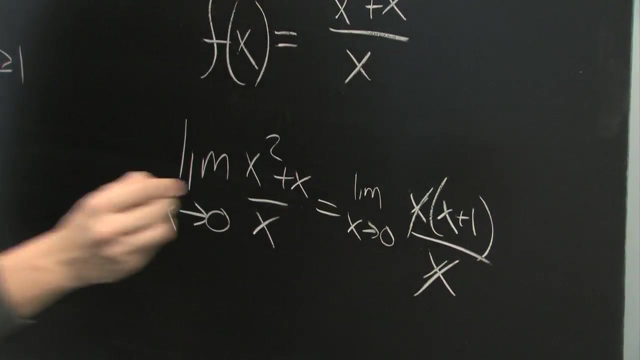 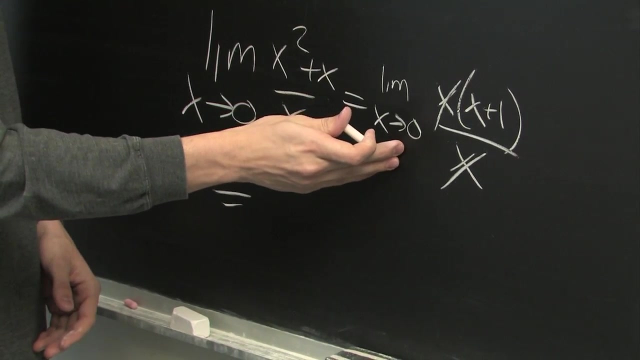 x. well, we can factor the numerator and we get x times x plus 1 over x. We can cancel out the x in the numerator and the denominator and what we're left is the limit, as x approaches zero, of x plus 1, which is simply one. 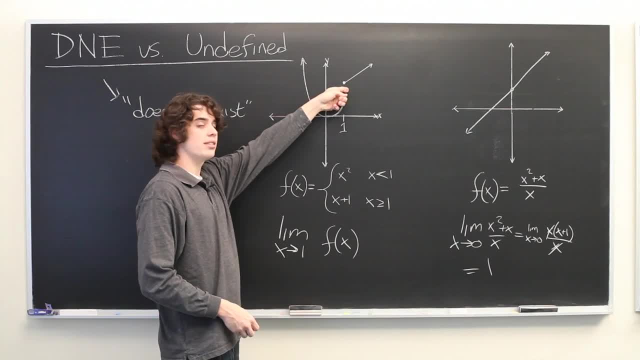 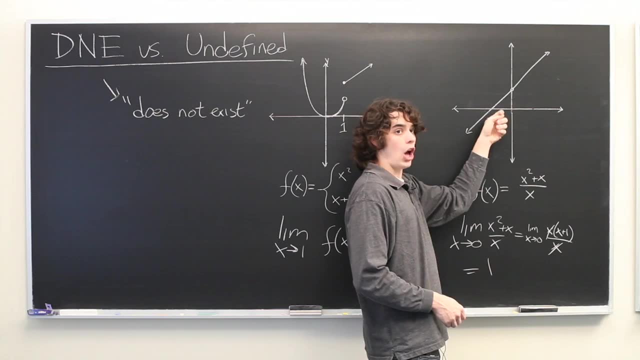 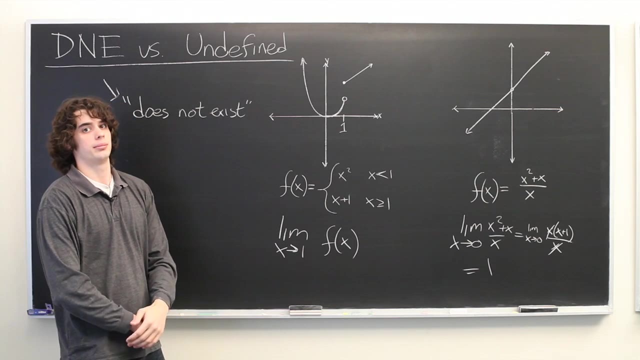 to recap, here we have a function that is defined at a point, but the limit does not exist, And here we have a function that is undefined at one point, but the limit does exist. As you can see, the two terms are not equivalent. My name is Ryan Malloy and we've 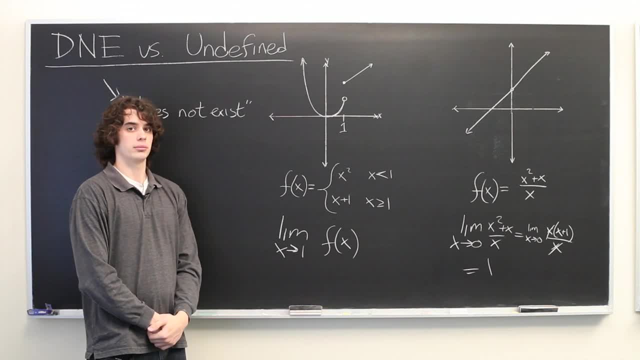 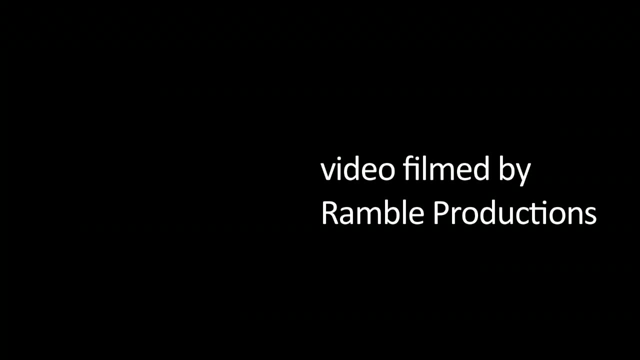 just discussed DNE versus undefined. Thank you,